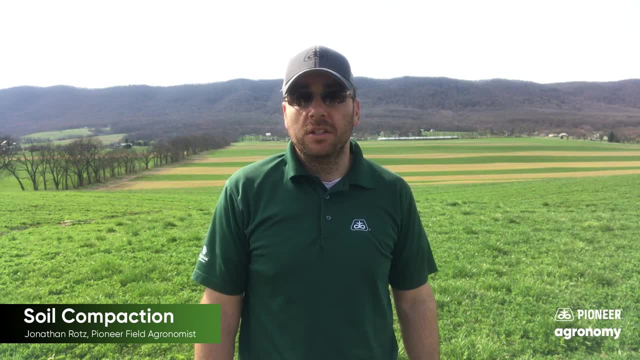 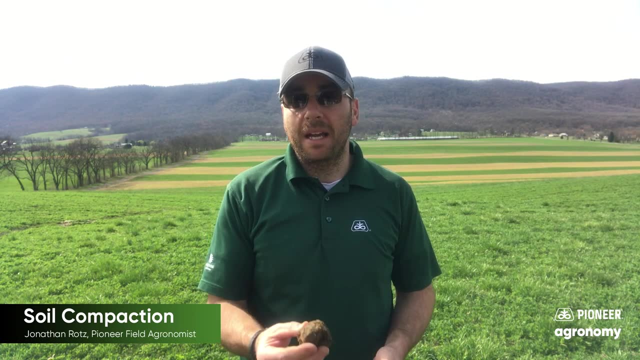 things. We'll get into spring forages here before long as well, And just a good time to review a little bit about compaction. One of the first things I always like to talk with guys about compaction is to really pay attention to the soil. So when we think about compaction, one of the first 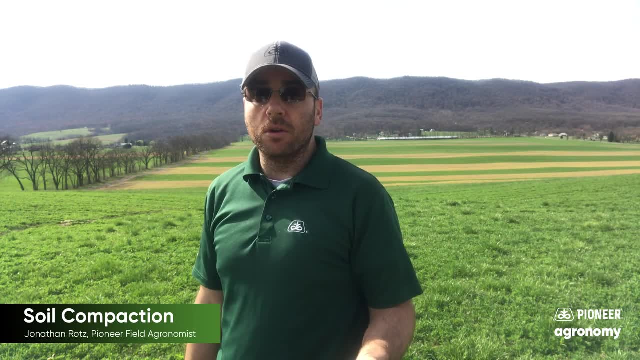 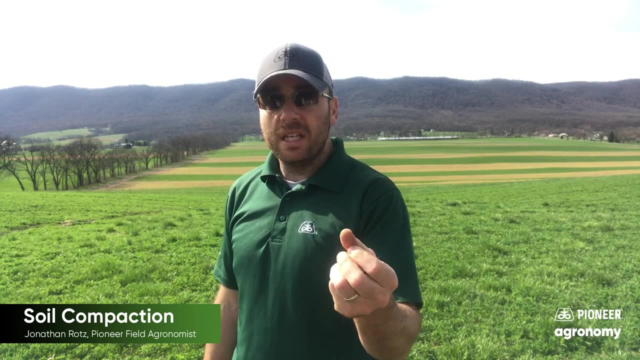 things to think about doing is going out and actually getting a little bit of soil. There's two different ways that we can look at compaction. One is the ball method, where we simply go and squeeze that ball And if we can dent that ball without really having it crumble around, 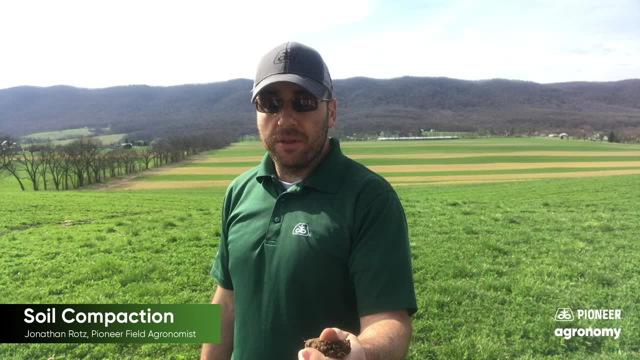 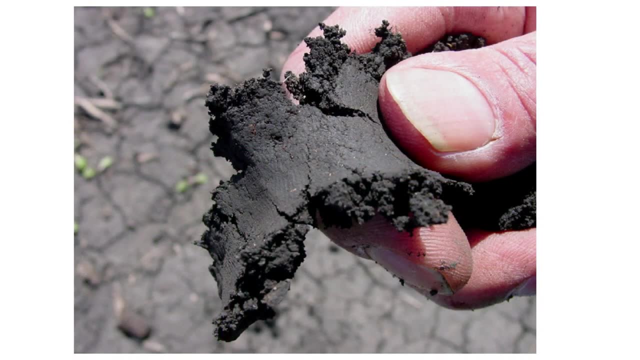 that soil is too wet to be on. The other would be the ribbon method, where you can push that over Your fingers, And if you come down two fingers, this one's actually probably not going to work very well, because there's a lot of root mass in here. But try to get yourself a nice sample And 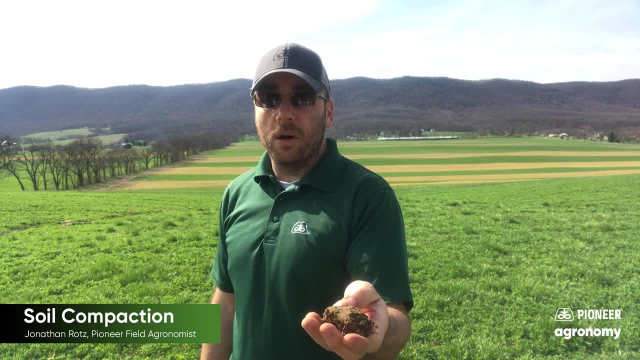 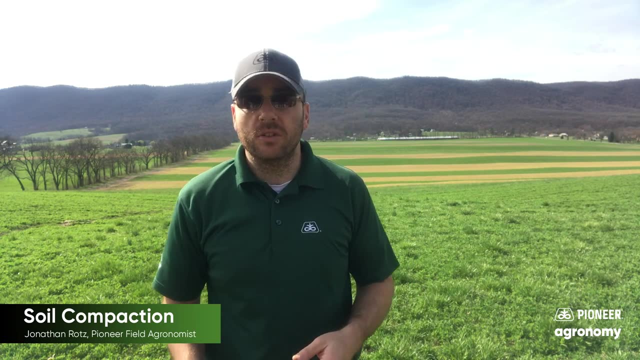 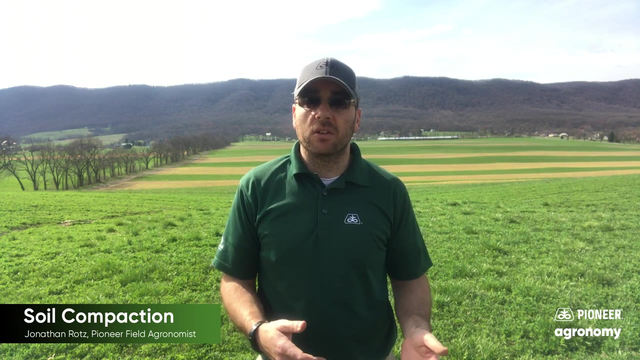 here, where I see that I'm not really cracking apart as I make that ball of soil again a little wet to be working on. Obviously, the reason I'm talking about wetness is wet soils increase our risk of compaction. Compaction is a serious thing, especially here in the spring when, if we're in 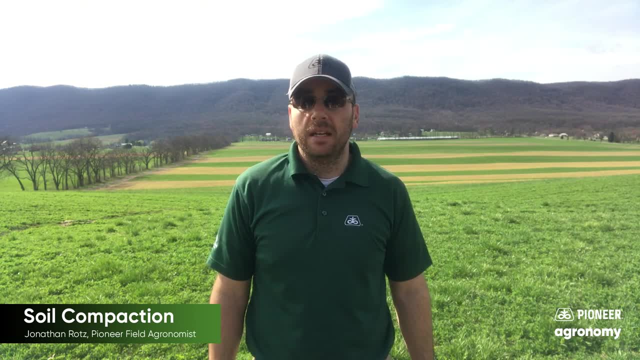 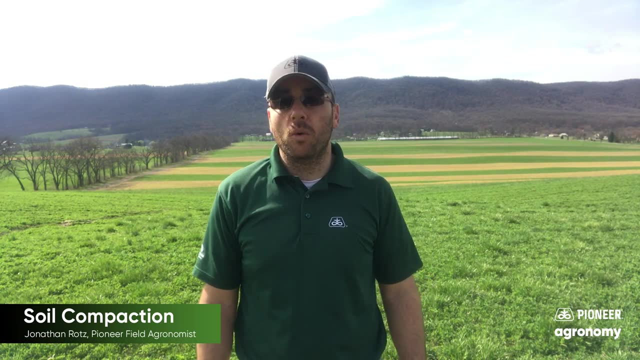 no-till scenarios, Especially maybe we're not going to have as much time to remediate, Or if we are in a tillage situation, as we go through and get our tillage done if there's anything else we don't want to. 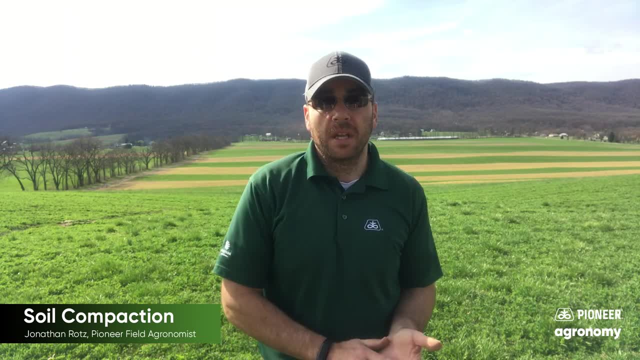 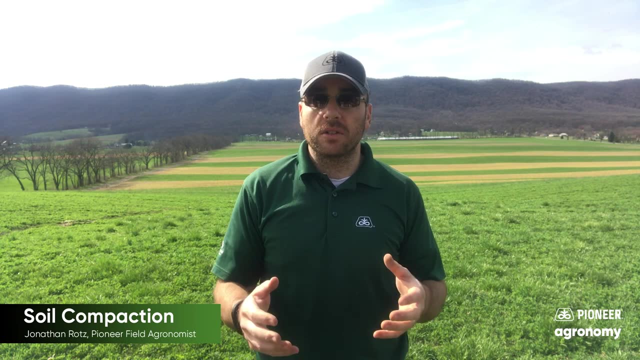 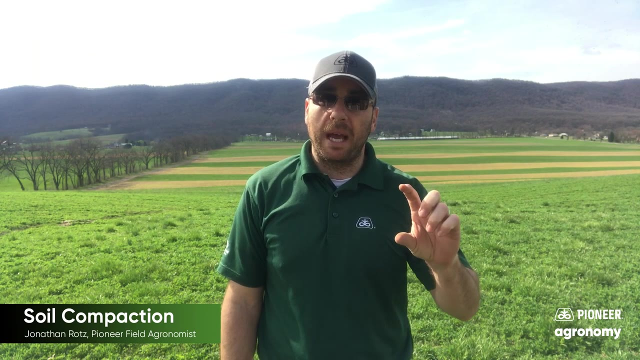 compact it prior to planting or during planting. One of the things to really understand about compaction is axle load. So we talk a lot about flotation tires and all of those kind of things which have a big play in compaction, But our flotation tires actually have a play on surface. 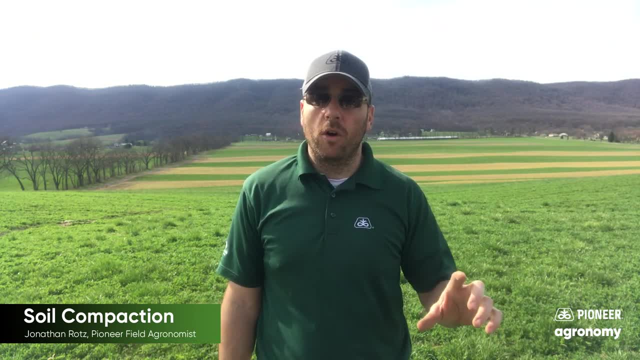 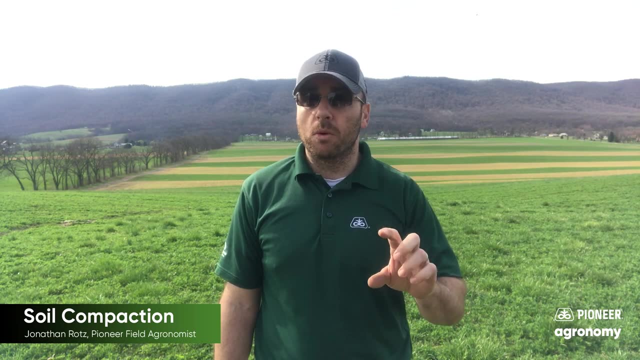 compaction. So the larger surface area of the tire, the bigger the surface area of the tire, the bigger the surface area we have on that flotation tire or whatever else. the larger area, the less pounds per square inch we're placing on that soil, the less we're going to compact that surface. However, our 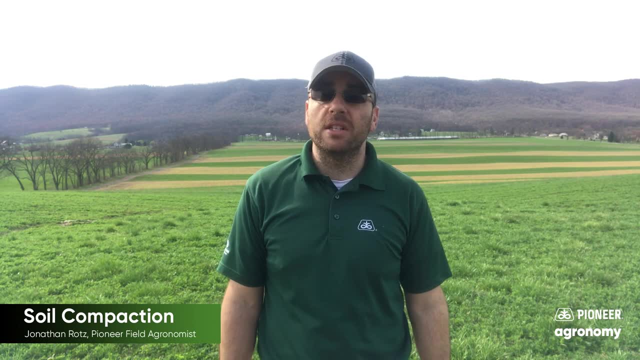 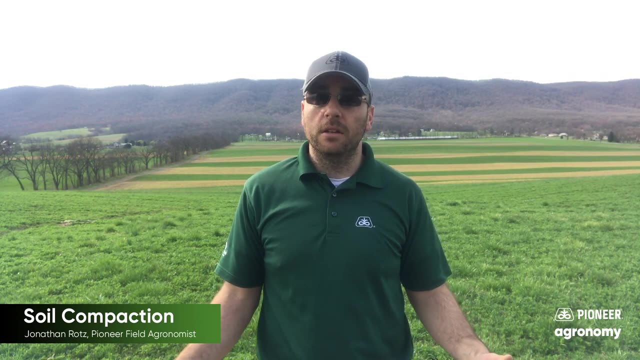 deep compaction that goes down into our subsoil is actually based off of axle load. So even if we put a large flotation tire on a really heavy load, we can still compact deep even though we're not compacting the surface Really. when we look at greater than 10 tons per axle is where we start to get concerned about. 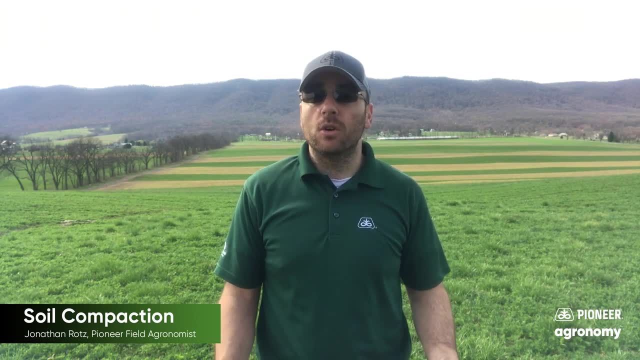 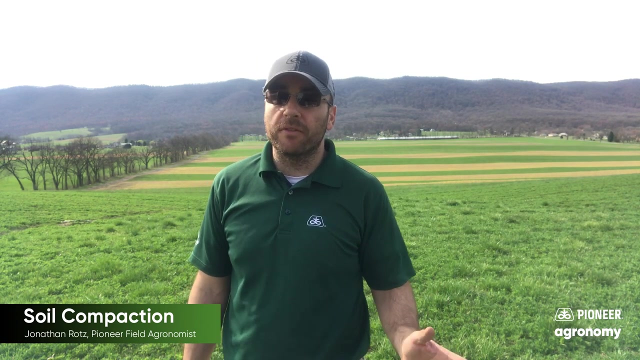 penetrating to that subsurface And again, as we get into wet conditions and things like is fairly typical of springs, especially the last few, we have more of a chance of getting that compaction deep. Another thing to think about is that 80% of your compaction is found to be on your first pass. 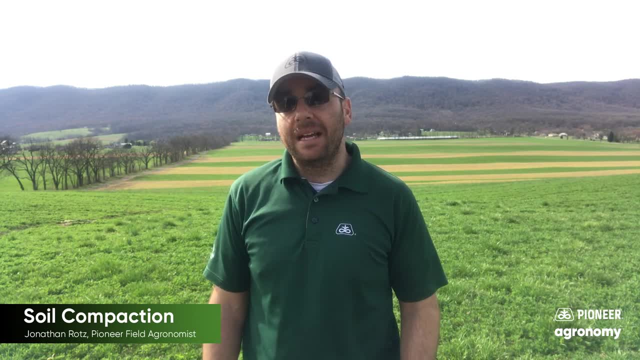 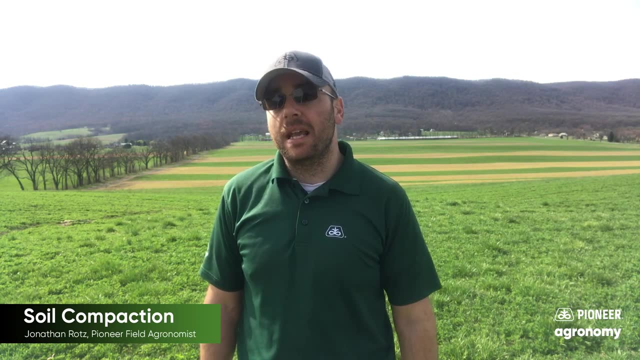 So this is why sometimes, if we're hauling manures or things like that, maybe making a path through a field where we go out and return on and just hitting that same path is going to be a better place. We are going to create some severe compaction in those areas. but there's two things. Number one: 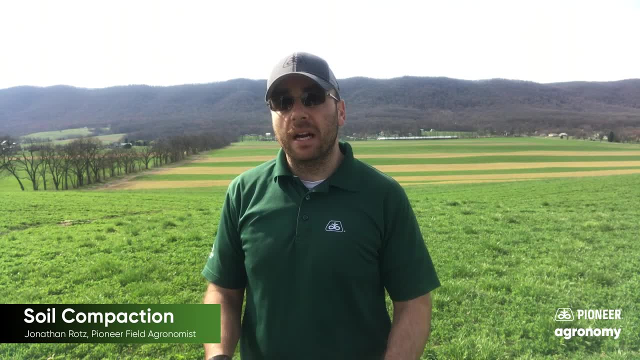 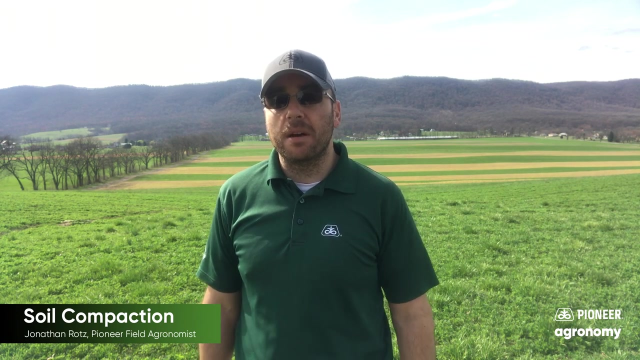 we are focusing that compaction in a small area. Plus, it's easier to remediate down the road without having to remediate across the whole field. So that brings me to the idea of what do we do about compaction if we get it there? Well, light to moderate compaction. a lot of times we think about 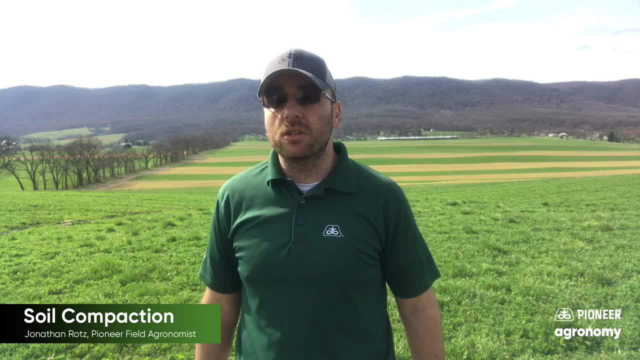 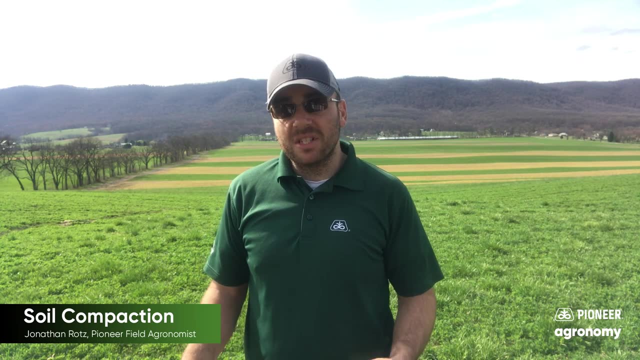 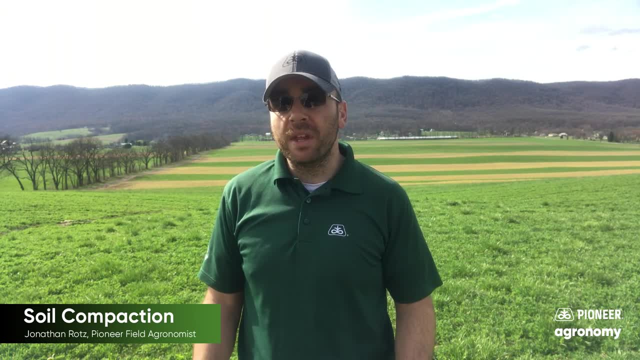 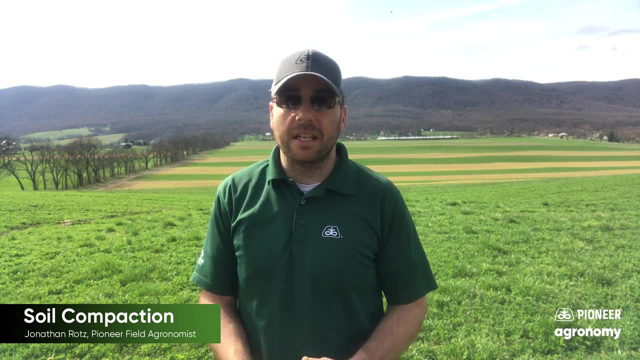 a lot of times will need some level of tillage. When we think about this, there's all sorts of tillages, You know. we think back about the moldboard plow- and I'm not a fan, obviously- and one of the things to think about when we think about tillage is: how does that implement? look across a plane. 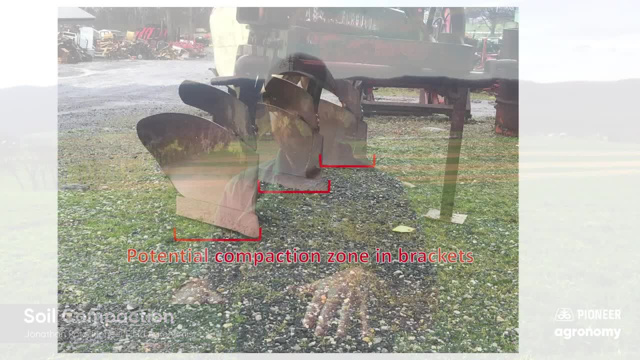 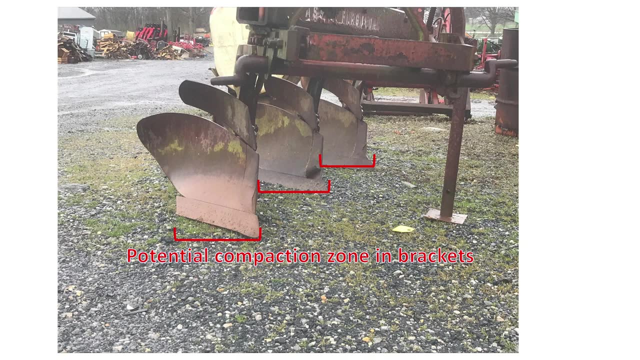 Let me show you a little example first. So, for instance, if you think about a moldboard plow, when you look at that straight on, you can see a line across that whole plow that's going to be smearing as you come across. That's where our plow pans and things like that get created. 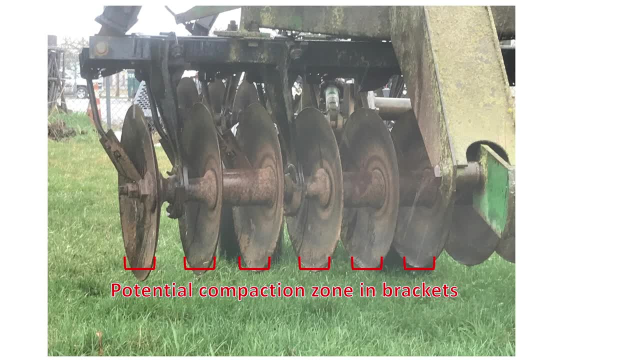 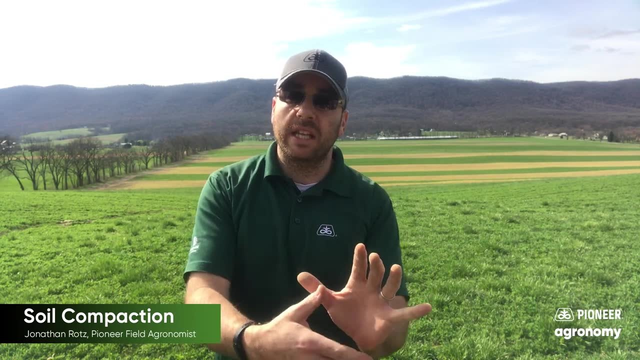 Disks- actually especially offset disks- tend to do the same thing. As we have those disks to the side and as we push them forward and move through, there's a lot of surface that is actually getting a piece of steel slid across it. There may be some gaps in the middle, but that surface still has a 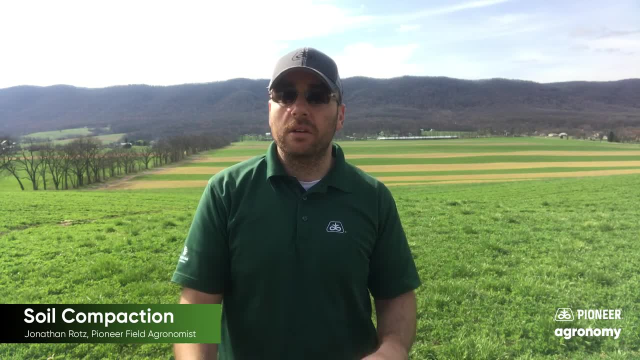 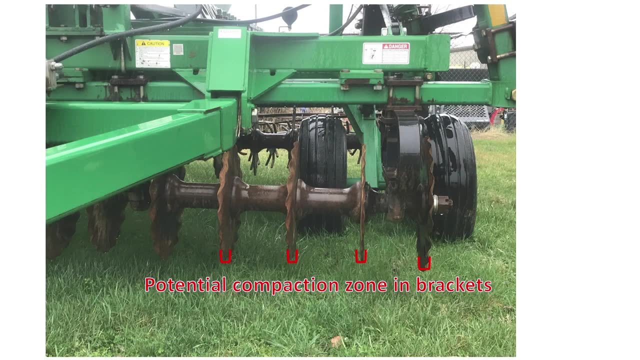 that gets slid across and especially if you're in a wet condition, we can create a pan and we've seen disc pans as well, some of our men till systems. you'll see when you look at that implement that there's a lot more space in between. so you know things, things along the line, when we think about.